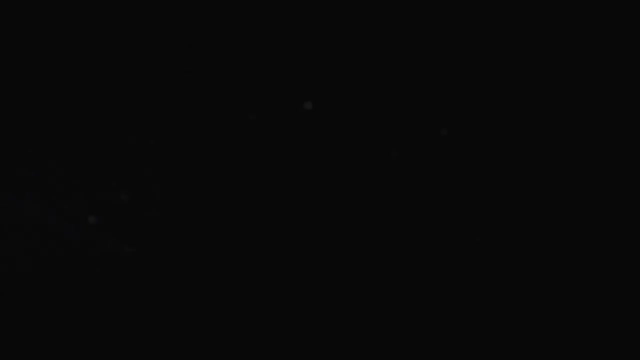 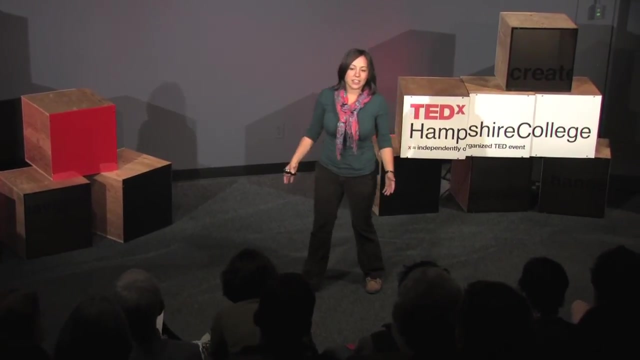 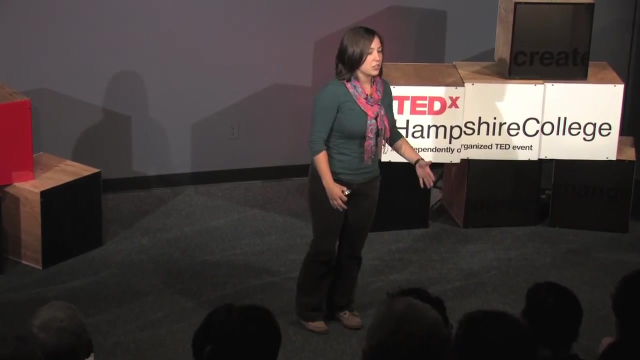 So the most interesting thing about the Continuum Hypothesis- although it has 8 million hits on Google, it's religiously interesting, it's philosophically interesting, but the most interesting thing about the Continuum Hypothesis is the light that it sheds on what we can and can't. 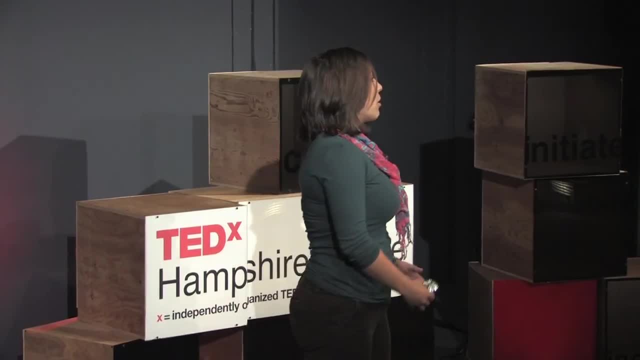 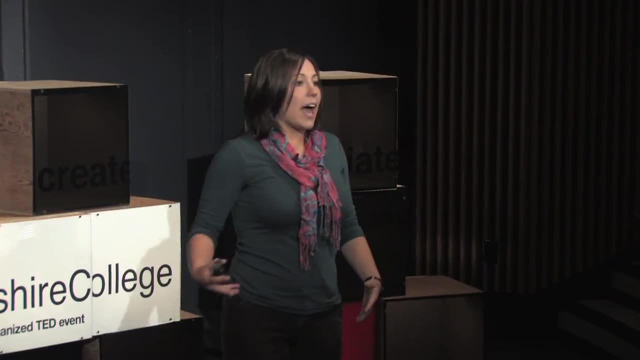 know in mathematics. So oftentimes cultures and people- probably many of you in this room- will turn to mathematics anytime you want a rational and decisive answer when your economics or your philosophy can't give you that answer. Galileo said that the universe cannot be read. 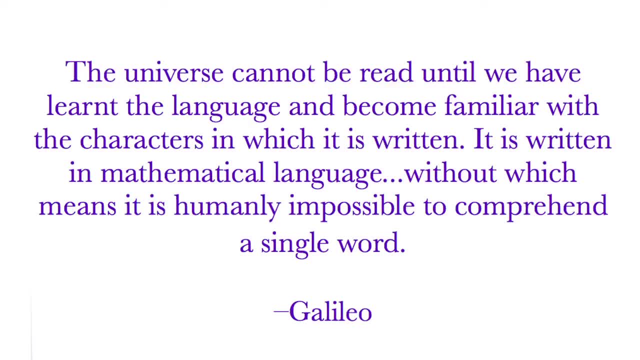 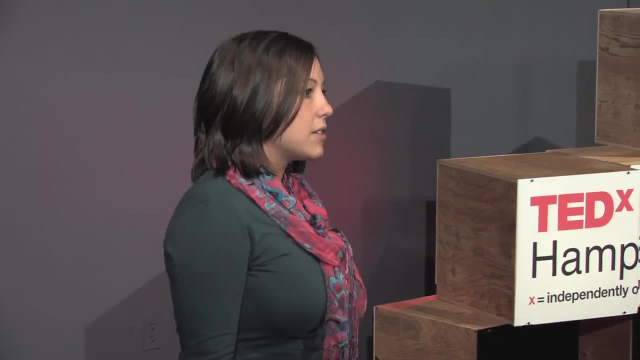 until we have learned the language and become familiar with the characters in which it is written. It is written in mathematical language, without which means it is humanly impossible to comprehend a single word, So we often rely on these mathematical foundations to understand just about anything, especially in a scientific way. 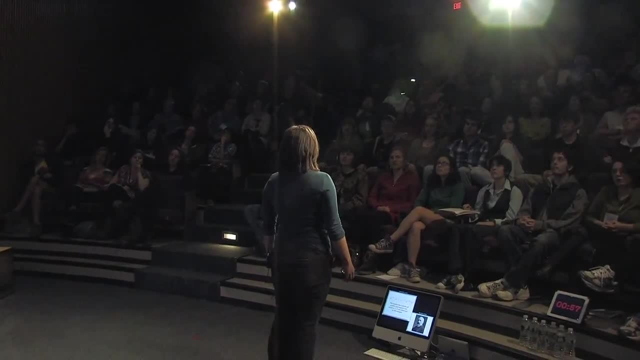 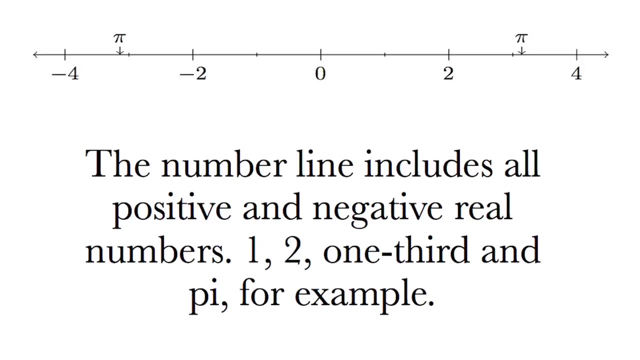 The Continuum Hypothesis is a simple statement about the number line. The number line, the one that we learned about in 3rd grade. It starts in the middle, it has 0.. It extends out to infinity on both sides. It includes all of the numbers, both the counting numbers- 1,, 2,, 3, and it also includes 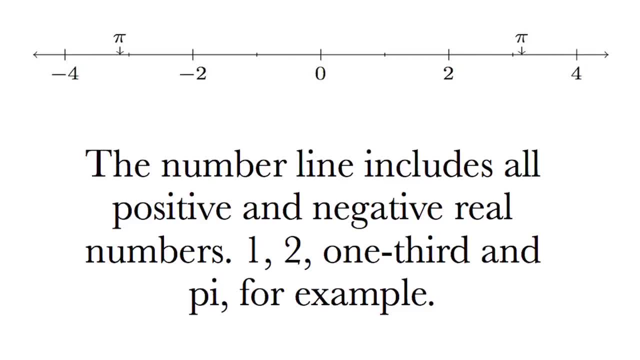 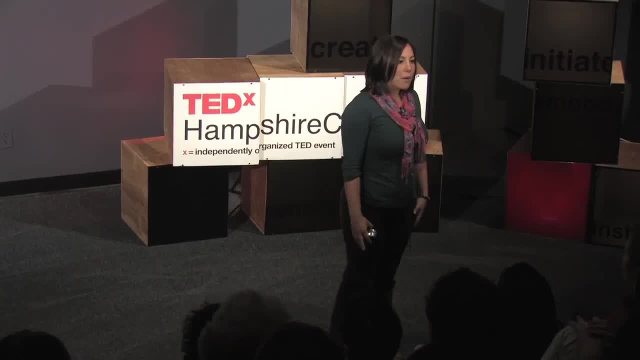 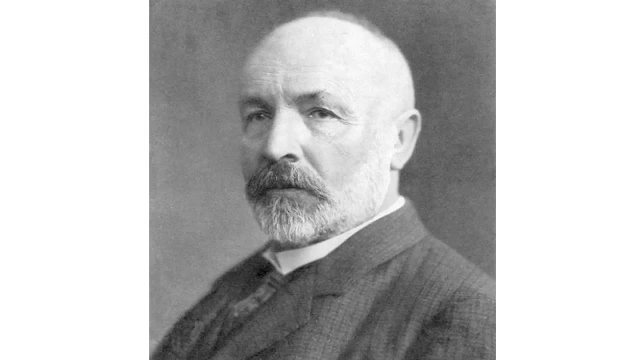 all of those numbers which take infinitely many decimal places to describe, Pi is one that you all are familiar with. The first person to ever think about what happens at the end of those lines, though, beyond those arrows, was a man named Georg Cantor. He was a German mathematician. 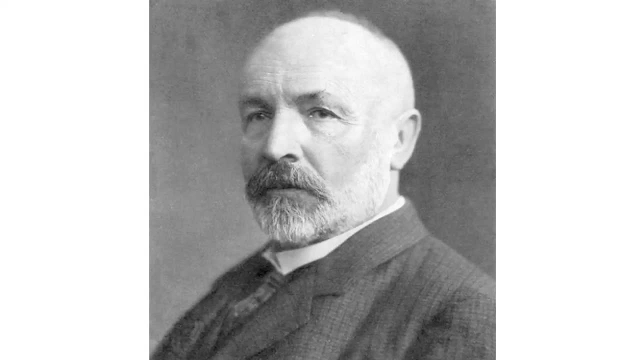 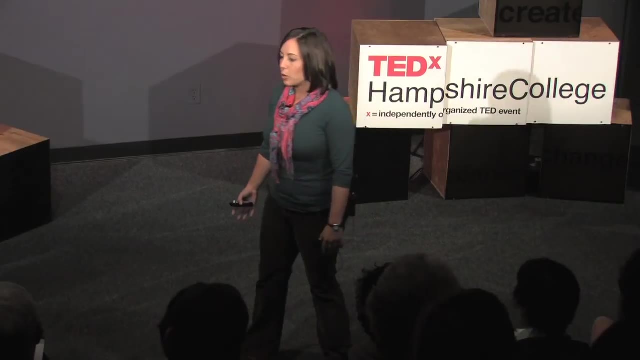 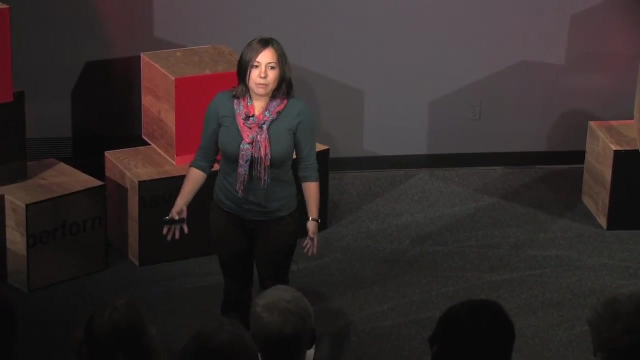 He developed these mathematically rigorous ideas of thinking about completed infinities. Before we had no conception of these completed infinities, and those of you who are familiar with calculus will know that we use infinity as limit points in calculus, and that was pretty. 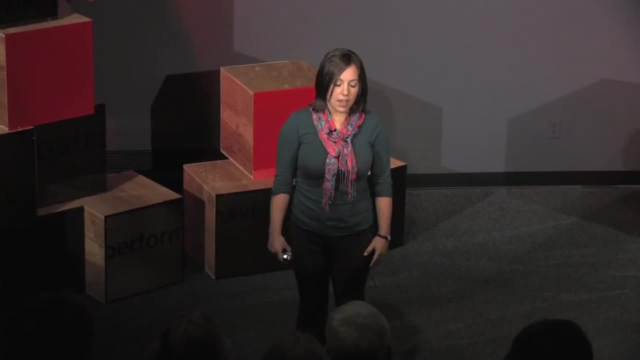 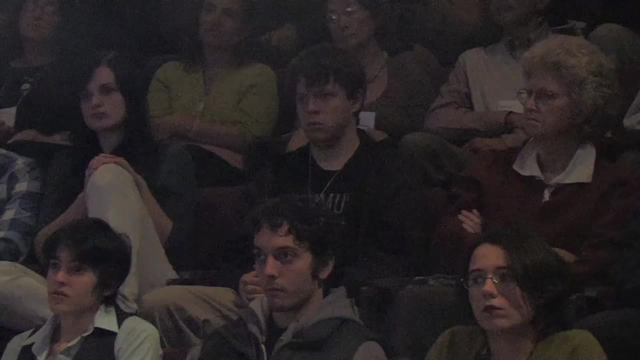 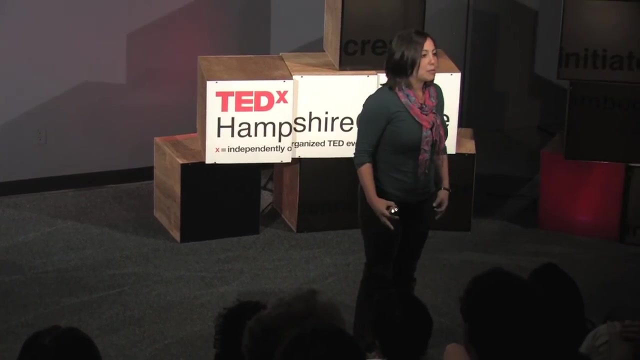 much the most rigorous way we had of thinking about any sort of infinity. Cantor, however, developed these ways of thinking about these actual sets of infinity and he developed ways of thinking about infinitely many of these completed infinite sets. He was met with a lot of skepticism, though. Cantor was a Jew and the most famous mathematician at the time. 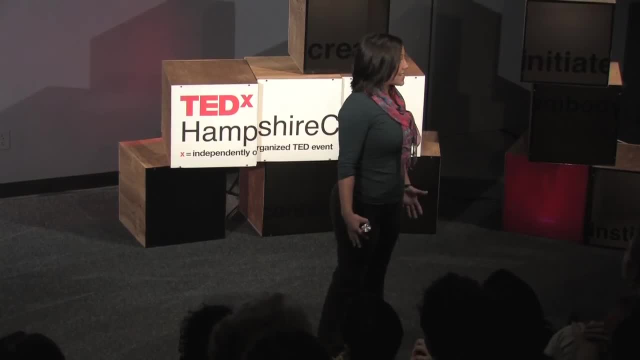 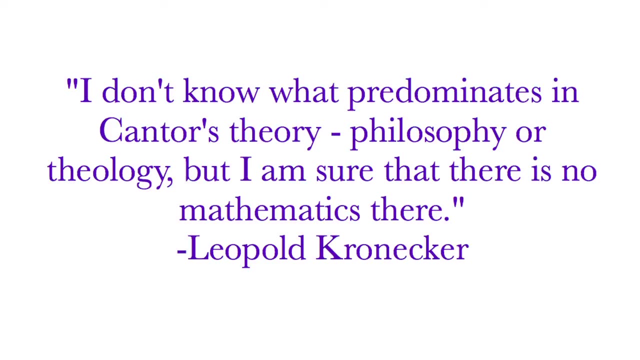 in Germany. his name was Leopold Kronecker. he was a known anti-Semite. He said: I don't know what predominates in Cantor's theory, philosophy or theology, but I am sure that there is no mathematician. It was particularly a blow-blow on Kronecker's part, because he was perpetuating these ideas of a Jewish mathematics, that Jewish mathematicians were somehow different than Christian mathematicians. This was a reason he got the religious community involved and Cantor never achieved any position. 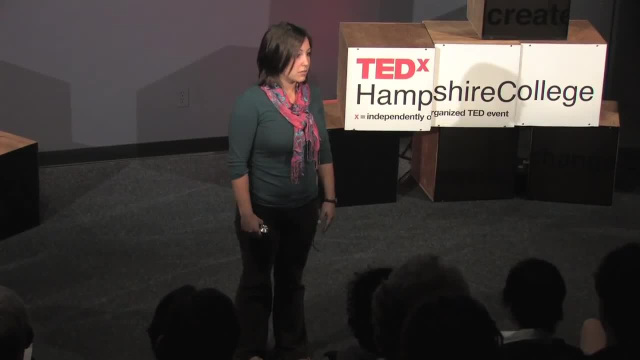 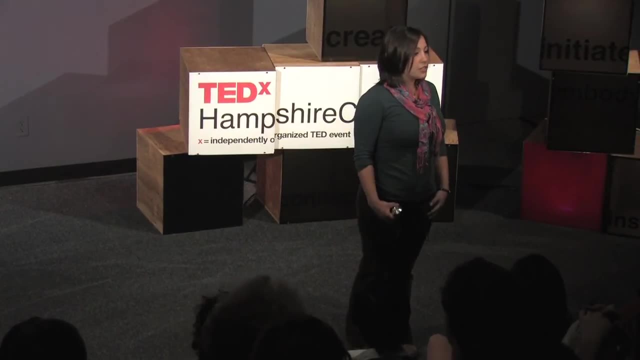 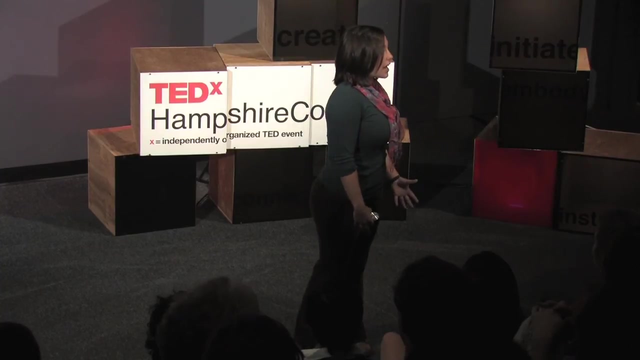 of merit. even though his ideas completely revolutionized fields of mathematics, Cantor wasn't discouraged though. Cantor pressed on, He developed a way of comparing sizes of infinity. So if we think about it at the finite level, if I want to know if the set of shoes that I have and the set of feet that 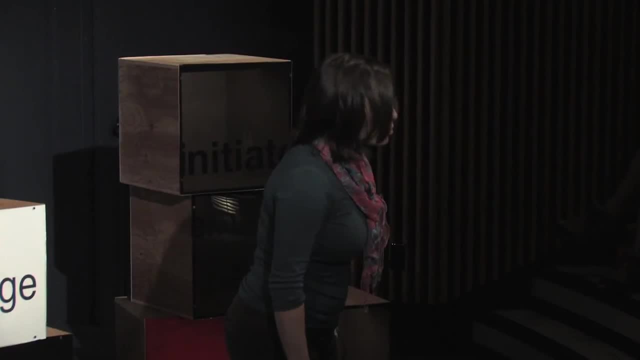 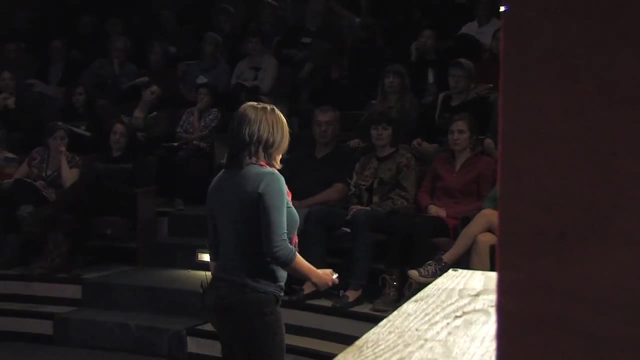 I have are the same size. I'll say: well, I want to put a shoe on every foot, and if I don't have any shoes left over, then I have the same number of shoes as I have feet. Well, Cantor applied this same idea to the infinite. So my claim to you is that there are actually 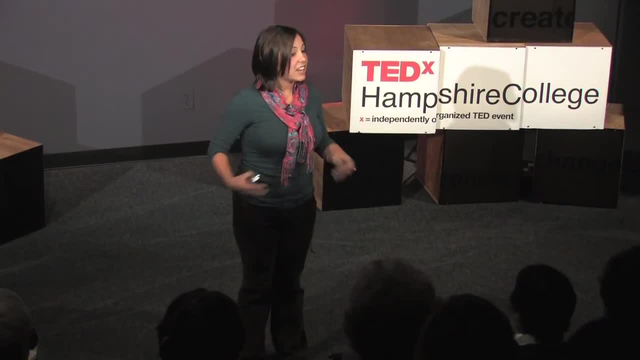 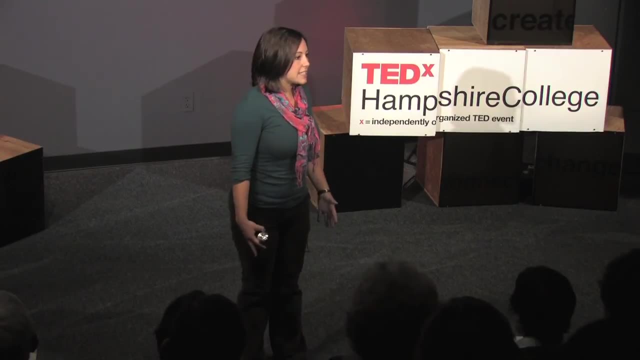 more real numbers. Those are all of the numbers that we're talking about here. They're not the numbers which take infinitely many decimal places to describe. Then there are natural numbers, the counting numbers: one, two, three, four, five. So some of you might say, well, 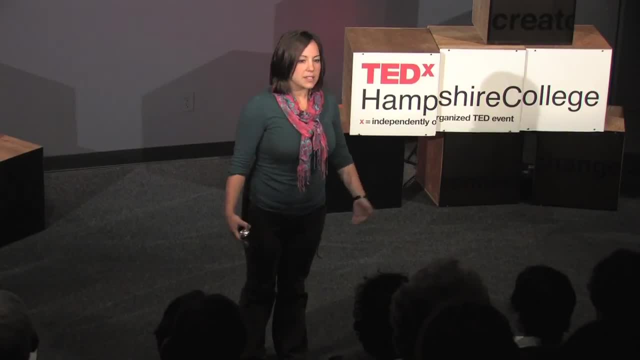 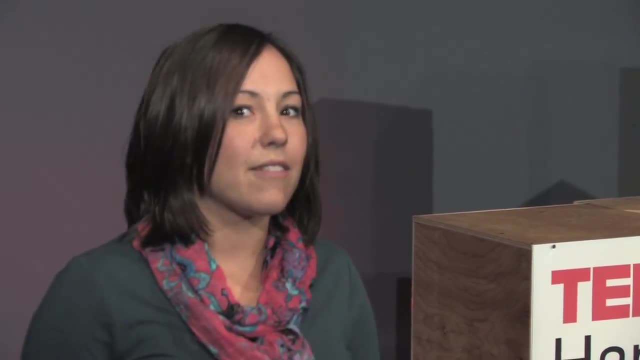 of course, there are real numbers in between, all the natural numbers, And then some of you might say: but both of them are infinite. How could there be more than the other? I'm going to show you a proof and I want you to use that same idea of the one-to-one correspondence. 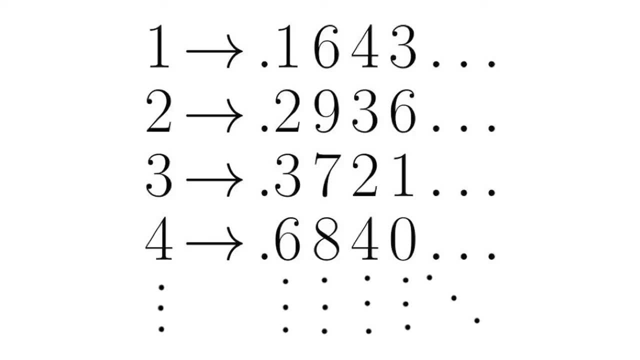 in this proof. So I want you to pretend like we can have this one-to-one correspondence between natural numbers and the real numbers. I've just listed some random ones there, but you can imagine, Imagine that there would be any of them, And then in your brains I want you to circle. 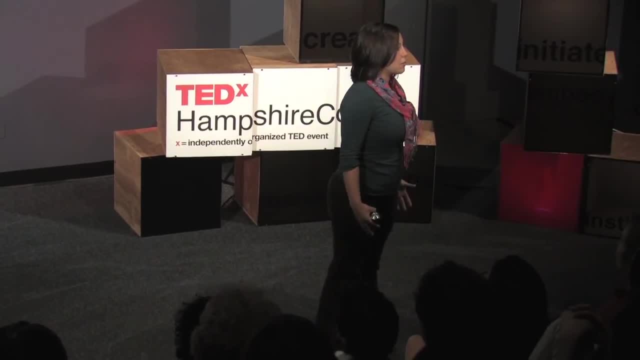 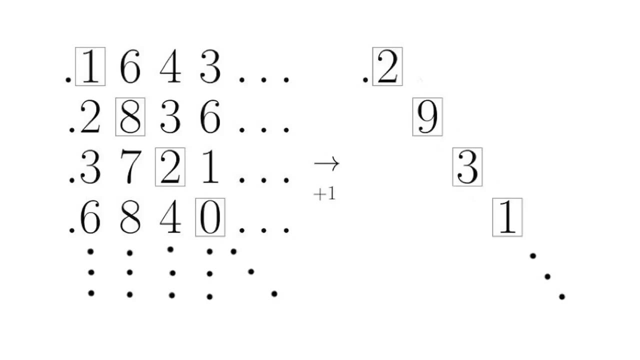 the first digit of the first number listed, the second digit of the second number listed, and so on. I want you to add one in your brain. to every single one of those numbers that you just circled in your head, We get a new number. We call it the diagonal number. It's: 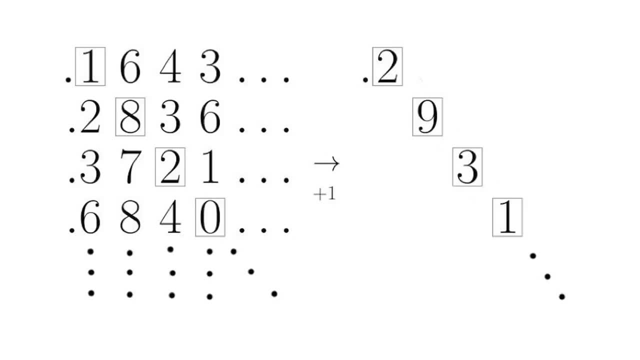 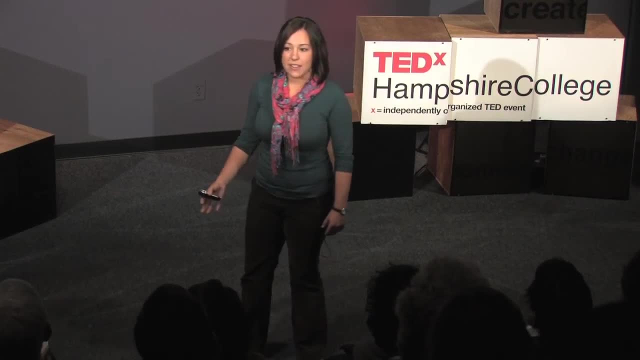 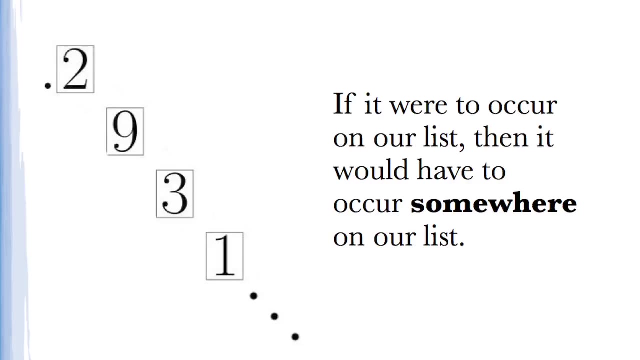 that one going down the diagonal. So it's the 10,000th digit of the 10,000th member on our list. And if it were to occur on our list- remember we said that we had included all of the possible real numbers- it would have to occur at somewhere on our list. It would have to have some natural. 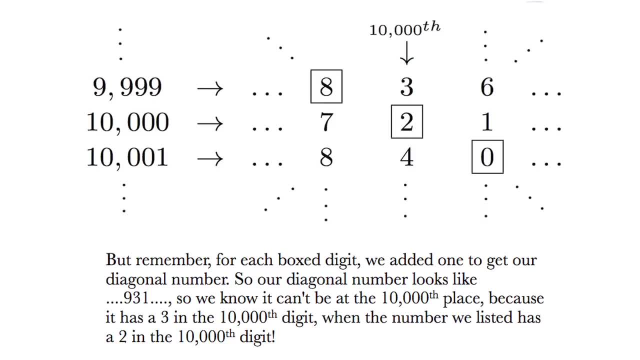 number corresponding to it. So let's say it was the 10,000th place. Well, we know that we added one to the 10,000th number we listed at the 10,000th digit in order to get our diagonal number. So we know. 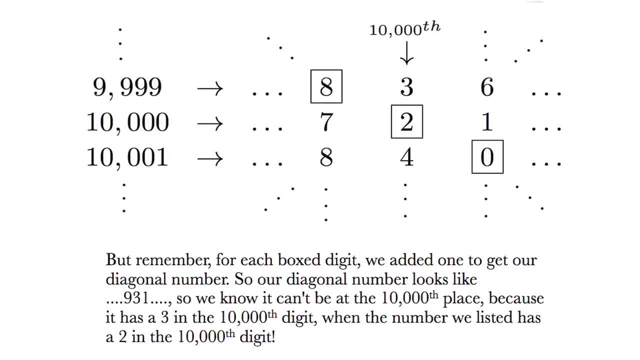 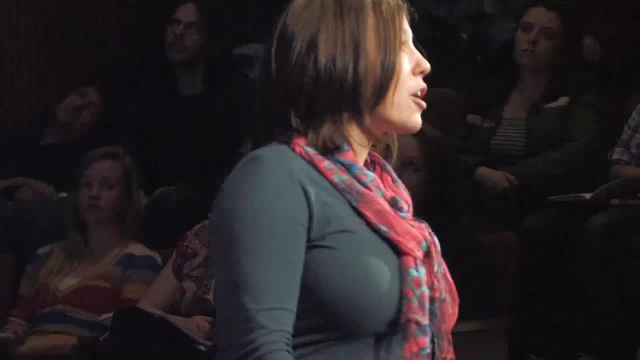 that it differs exactly at the 10,000th digit from the 10,000th number that's listed. So it can't be on our list. It can be nowhere on our list. So we have this number that's not on our list, even though we assumed that we had listed all of them. So now we know. 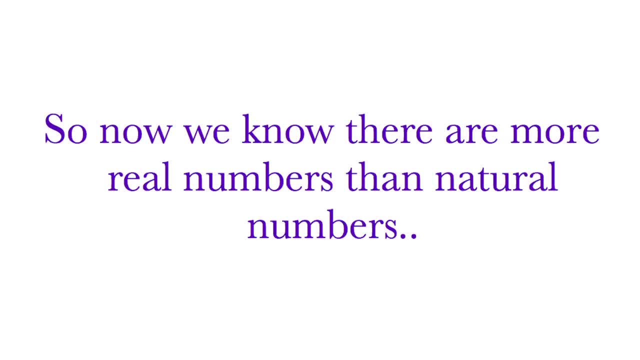 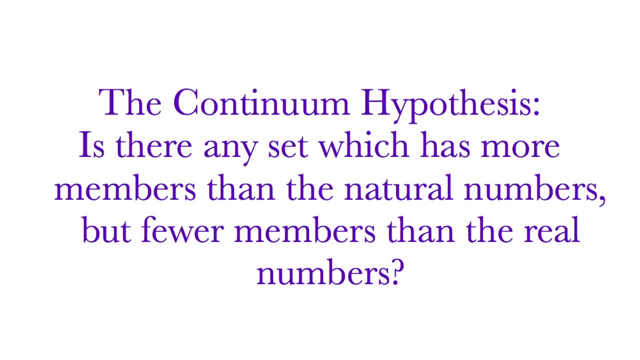 that there are more natural numbers than there are real numbers. If you didn't get that, don't tune out, You'll still get something from the talk. So the continuum hypothesis is stating nothing more than: is there some set which has more members than the natural? 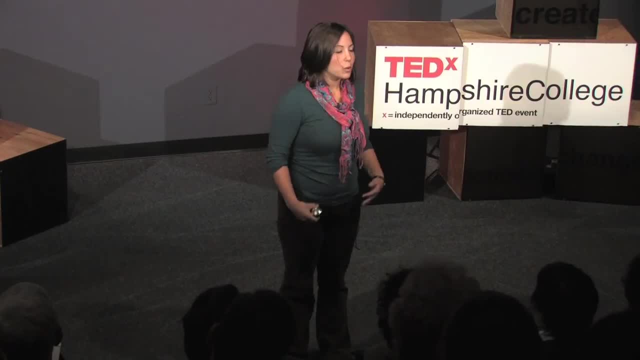 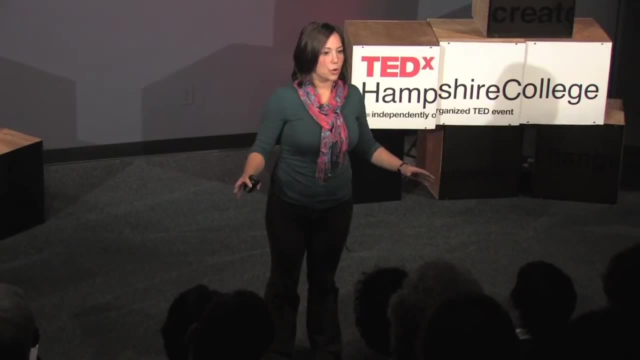 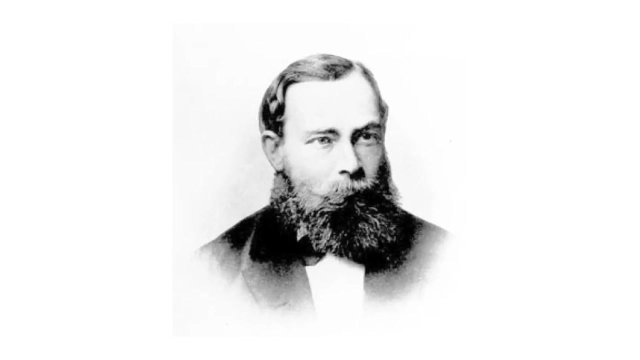 numbers and fewer members than the real numbers. It's a really easy statement to understand if you're familiar with Mathematica. So this story is sort of two stories. Cantor was doing his work in the late 19th century. We're going to meet another guy named Godleb Frege who is also doing his work in the late 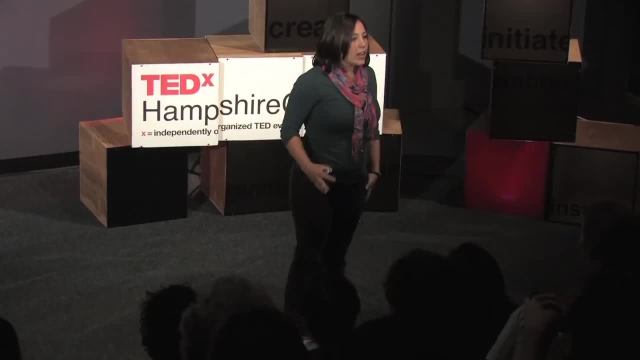 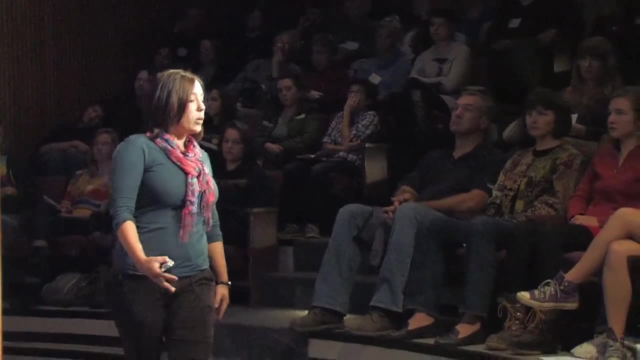 19th century. He was interested in a different kind of thing. Frege was interested in establishing rigorous foundations for arithmetic In geometry we have Euclid's postulates. We know a finite number of sentences for why everything in geometry is the way that it is. Frege was 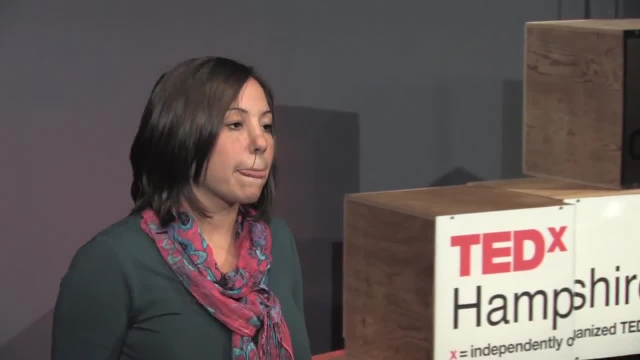 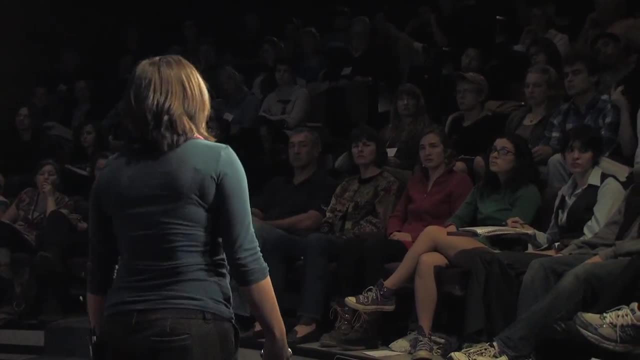 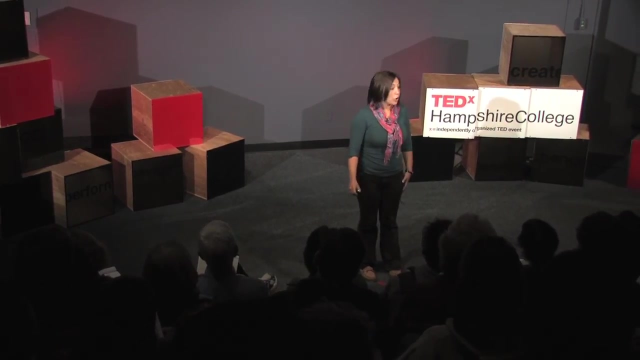 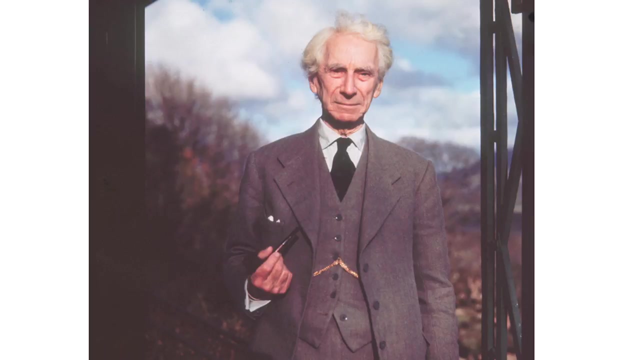 interested in a similar project for arithmetic. Frege published a book called The Basic Laws of Arithmetic. He thought that he had found a system for proving all statements of arithmetic. Sadly, in 1903 he received a letter from Bertrand Russell, an Englishman. Russell wrote Frege of a paradox that he had found in his system. 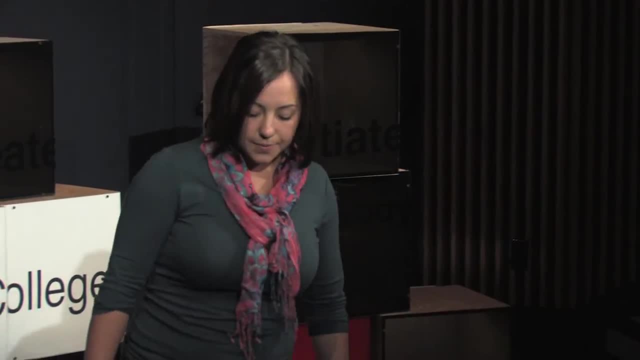 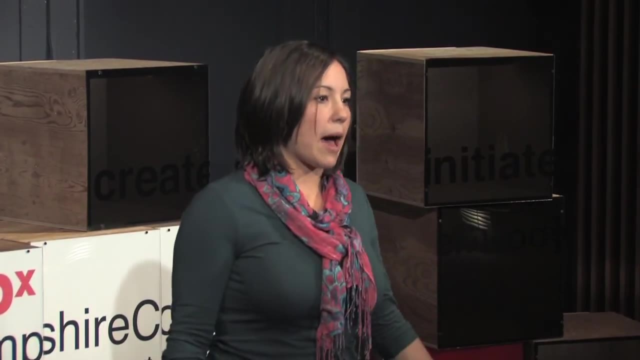 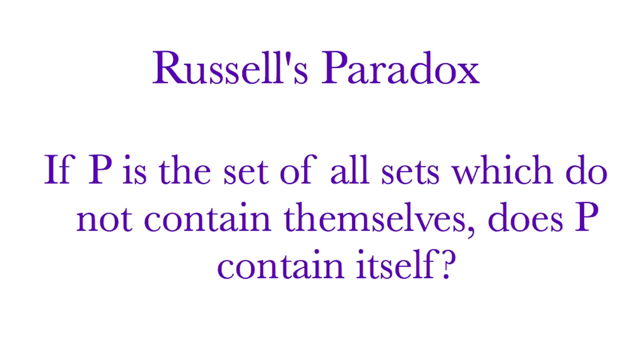 Some of you may be familiar with the paradox. It's called Russell's Paradox, And in Frege's system he didn't account for different sets containing themselves. He allowed for this to happen. Turns out this is not a good thing. Russell's Paradox asks if P is the set of. 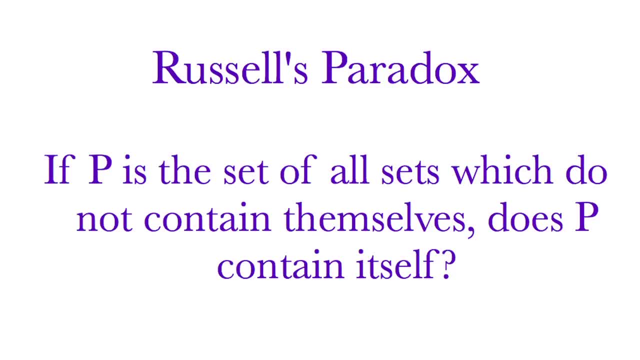 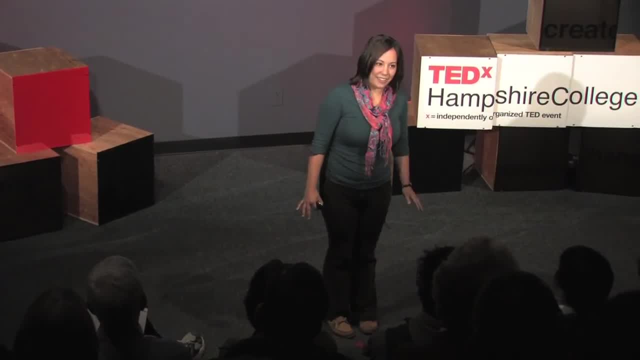 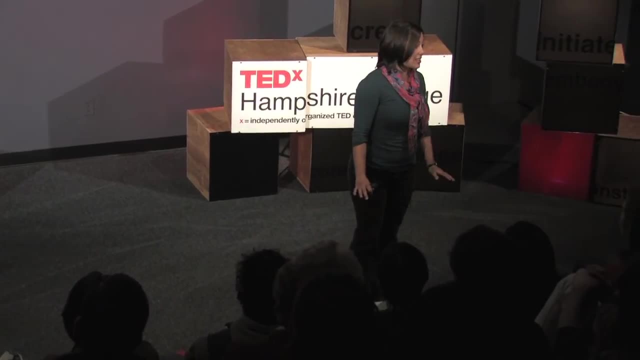 all sets which do not contain themselves. does P contain itself? So P would contain itself if, and only if, P didn't contain itself. A system can't really allow for these types of things. So this absolutely devastated Frege, He never was able to recover. He started writing some nonsense. I think he converted. 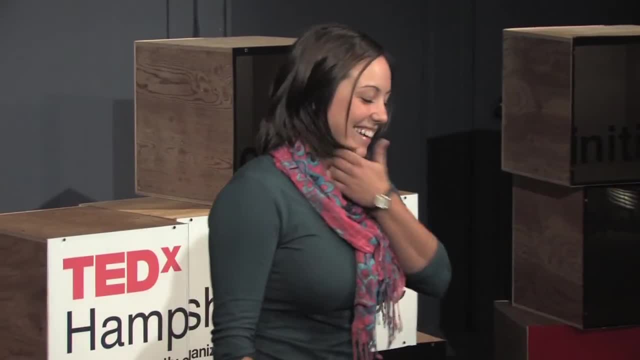 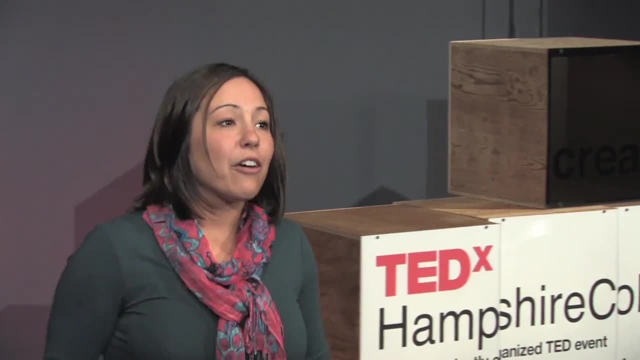 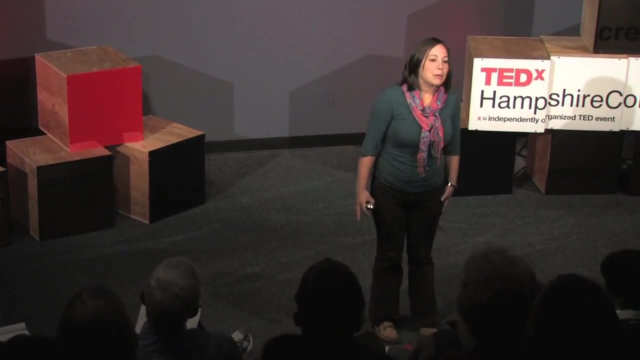 to Christianity after that. Anyway, Russell didn't give up on the project, though. He and a man named Alfred North Whitehead published what they called the Principia Mathematica. It's not Newton's Principia, But in this Principia it was two volumes and they were trying to figure out. 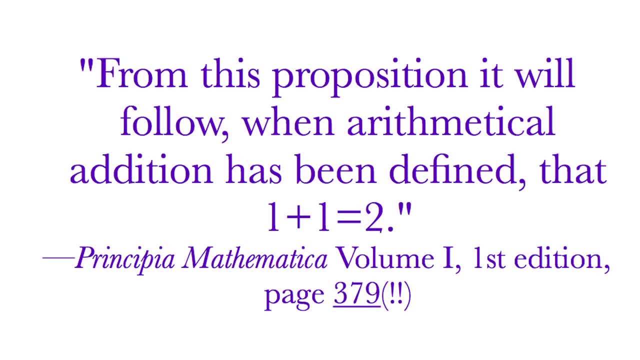 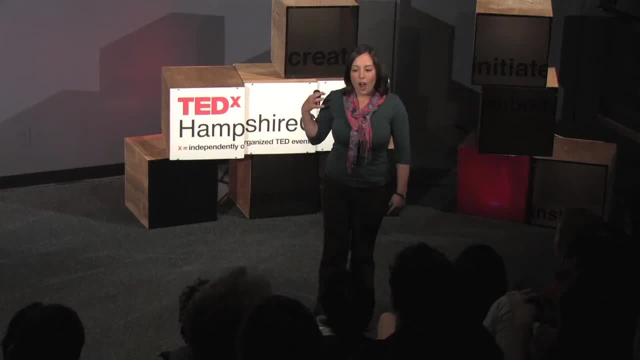 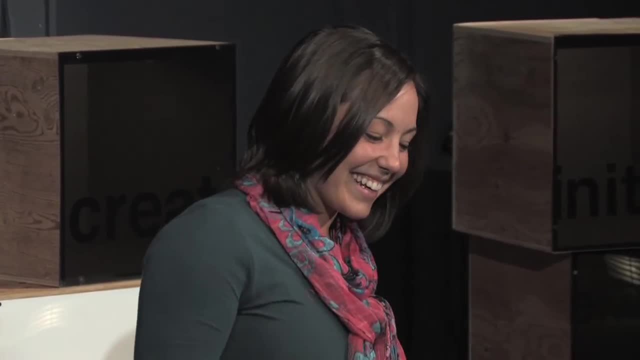 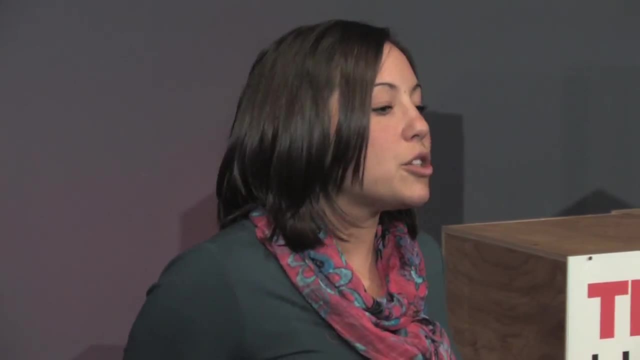 why arithmetic is true. On page 379, they proved that 1 plus 1 is equal to 2.. So they were leaving nothing up to intuition here. They really wanted a rigorous foundation. Laugh all you want, But after Russell they spent 12 years writing the first volume of this. They'd been so heavily 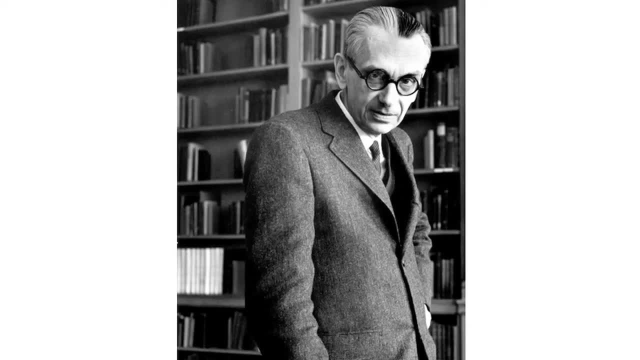 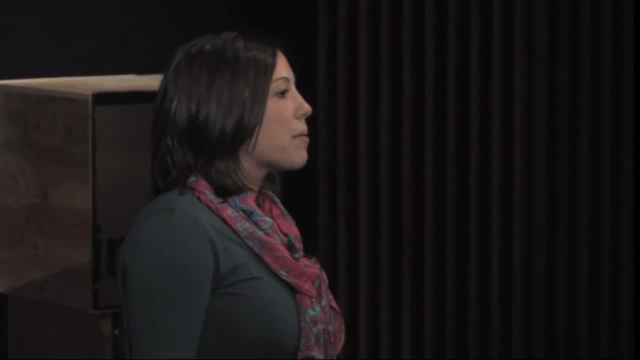 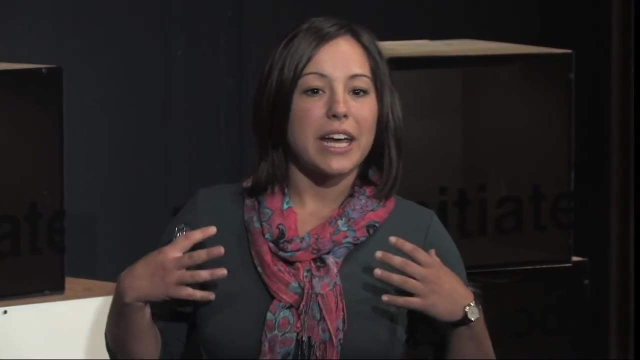 invested 26 years to do the entire thing, But a man named Kirk Riddell. He was able to prove. not only in Principia Mathematica was there a sentence of arithmetic that was unable to be proved, but for any system that could explain to us why arithmetic was true. 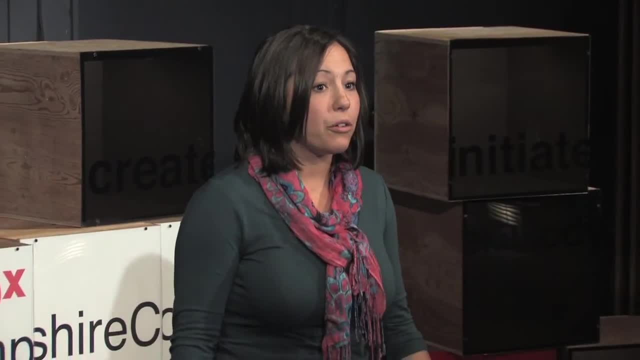 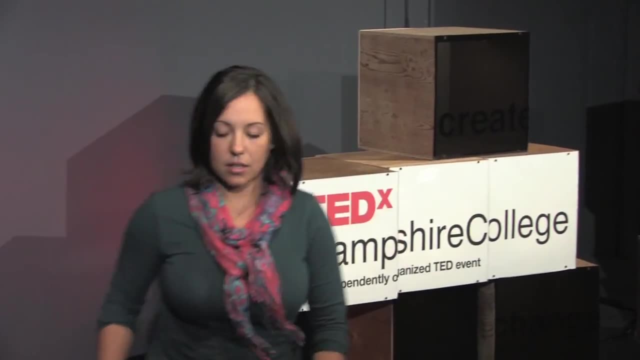 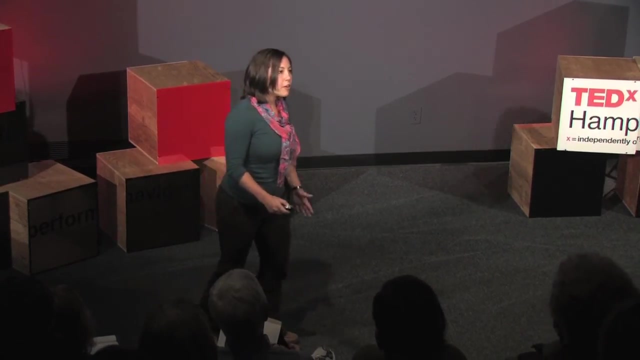 there's going to be some sentence of arithmetic that is neither provable to be true or false. So this absolutely destroyed Russell. He was not doing well when he read Gödel's paper, The sentence, though. it didn't bother other mathematicians so much, because the sentence looked something like: I am not provable in Principia Mathematica. So they asked the question like: why would we really ever want to ask if that thing is true or not? So they weren't too bothered. The algebraists kept doing their algebra and the analysts kept analyzing. 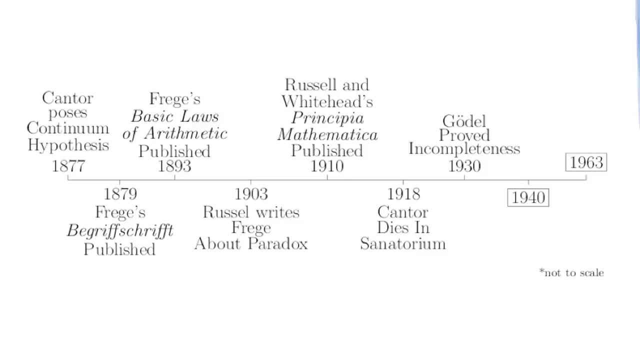 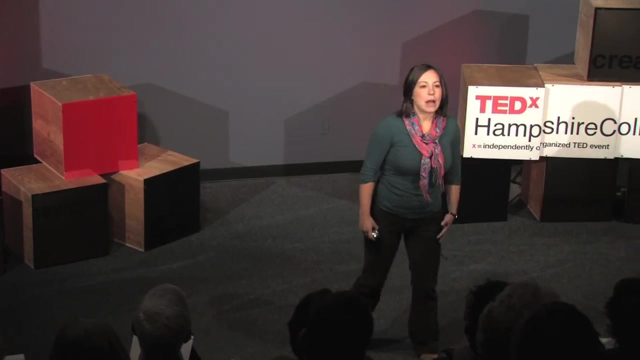 And while all this was going on, it's really sad Georg Cantor passed away. It's really a shame that he wasn't around in 1940, when Kirker did a really good job of telling us the truth. So Gödel, same dark horse, was able to prove in the simple statement of the continuum hypothesis: 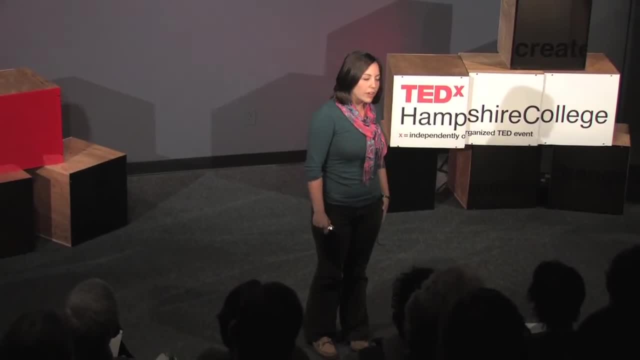 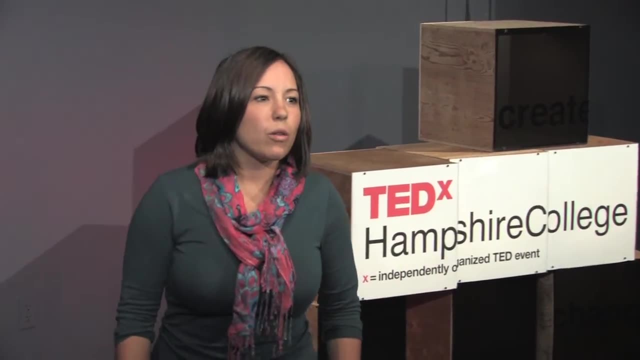 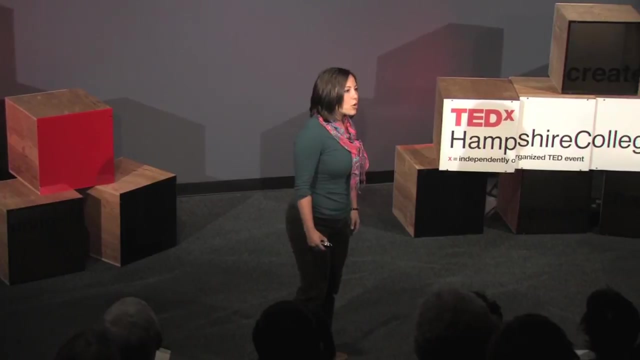 that we can't disprove it. So he didn't prove it. He didn't prove that anything was true. It was a new kind of proof and we proved that we would never know that it was false. So kind of confusing right, And no one made any progress on this. We had no new way of. 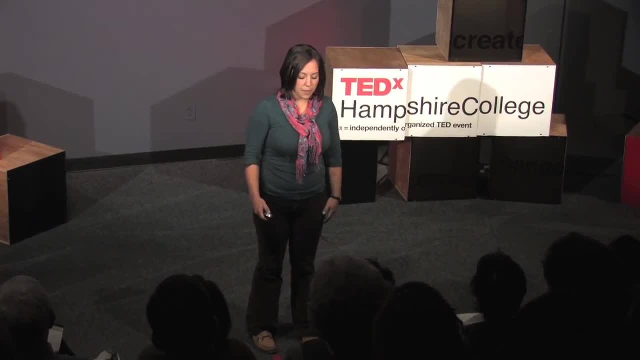 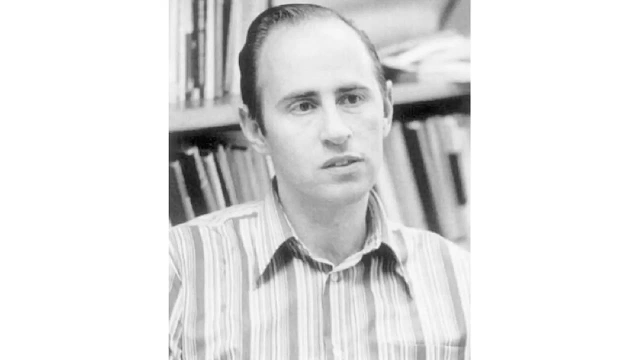 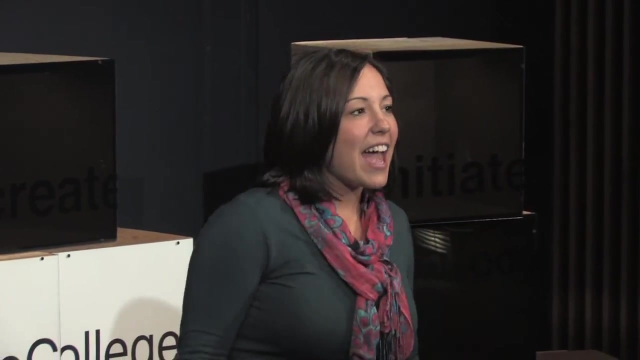 constructing proofs. in this way, Gödel sort of revolutionized this system, Until a man named Paul Cohen was totally hungry for power in the mathematical community And he was trained as an analyst. but he wanted to get famous And so he chose logic. He didn't think there were any smart logicians And he went up in the halls.